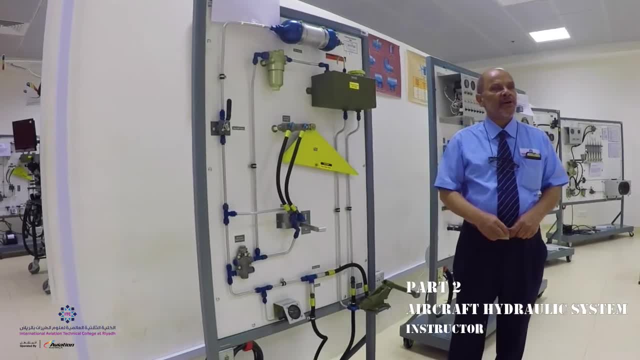 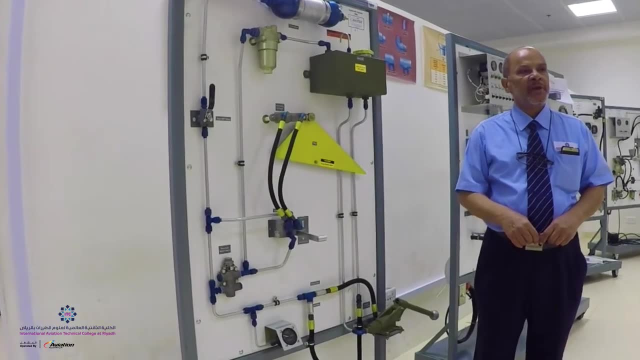 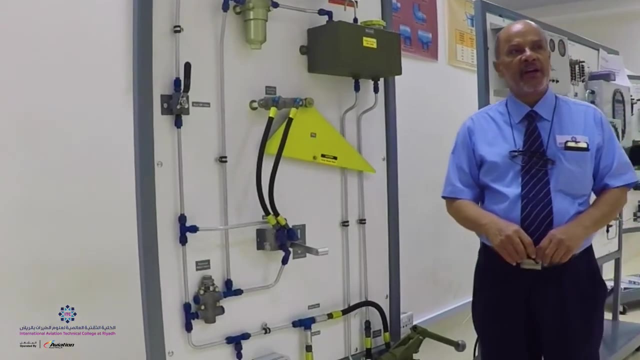 Assalamu alaikum, Welcome to IATC online training. On this session, we're going to talk about the aircraft basic hydraulic system. Before we start, I would like to mention a note about the importance of safety when working in aircraft in general, and especially when working with systems such as hydraulics. 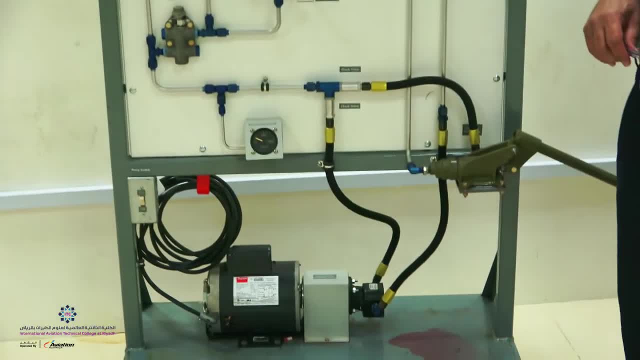 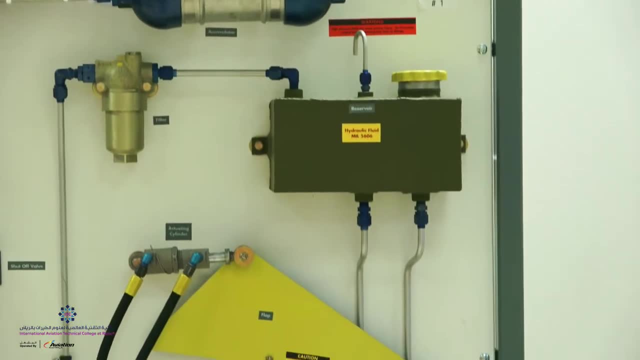 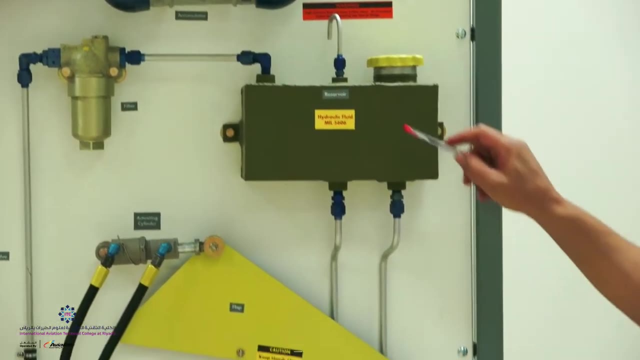 Safety always comes first when working with aircrafts. On the trainer, here we see the layout of the basic components usually found in the hydraulic system, Starting with the reservoirs, Therefore the tank that holds the fluid, the lines, as you see, the pumps. 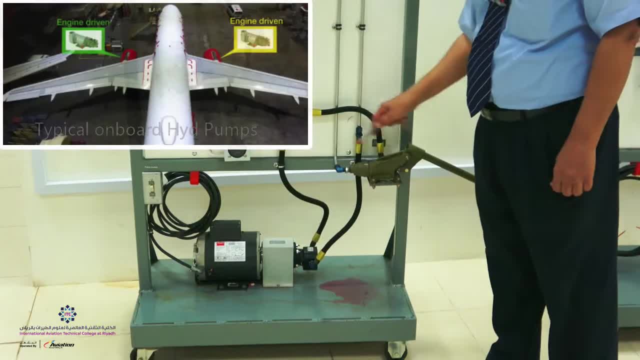 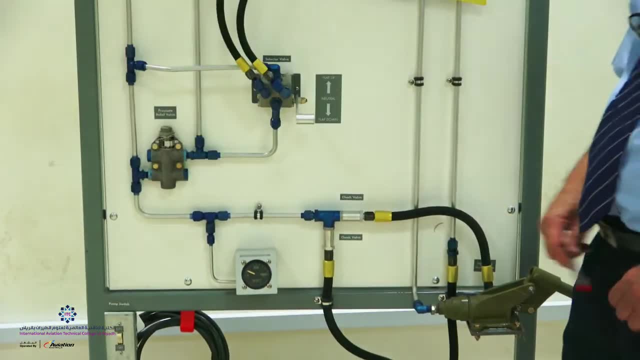 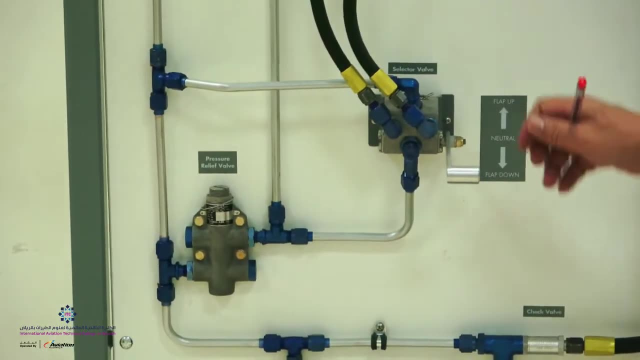 We have two types of pumps here. We have a manual pump and electric pump. We have gauges to measure system pressure protection in the form of pressure relief valve to relieve the excess pressure and a selector valve to operate the system. In this case, we have a flask. 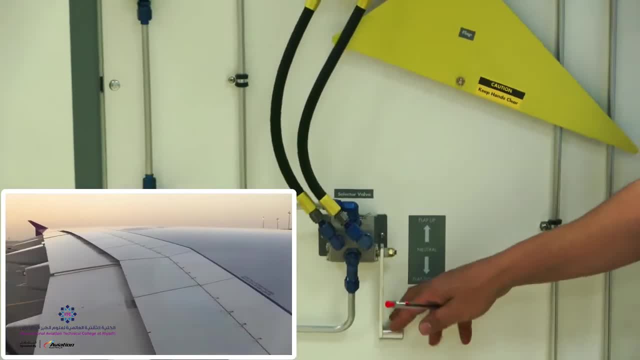 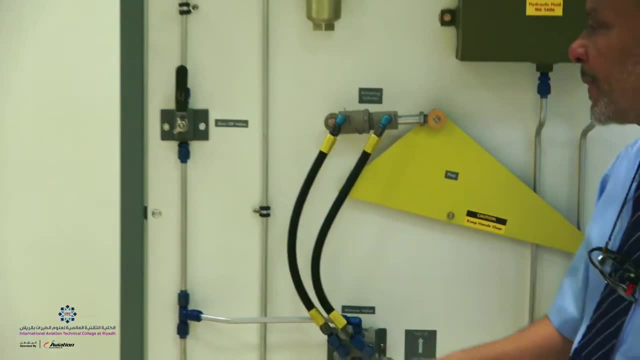 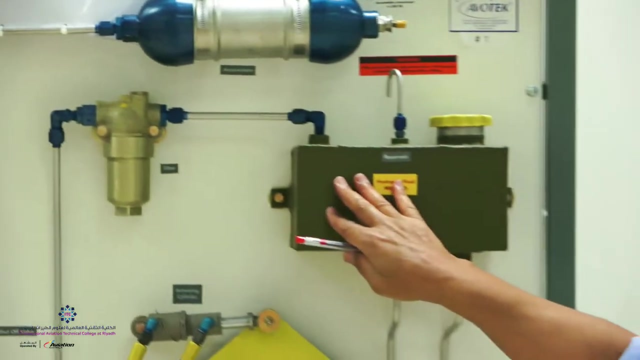 We have a flap shown here, a flight control named the flap, which will operate using the selector valve, the actuator that operates the flap, a shut-off valve to isolate the system. We have a filter to clean the fluid before it goes back to the reservoir. 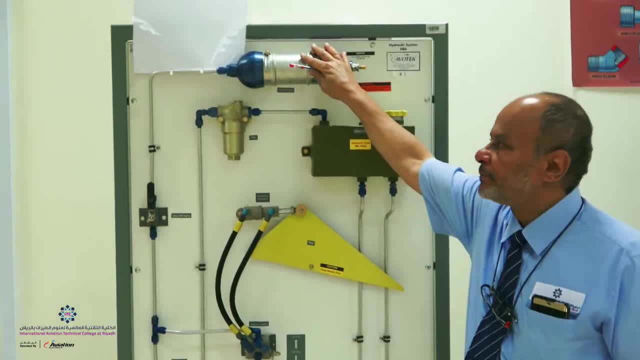 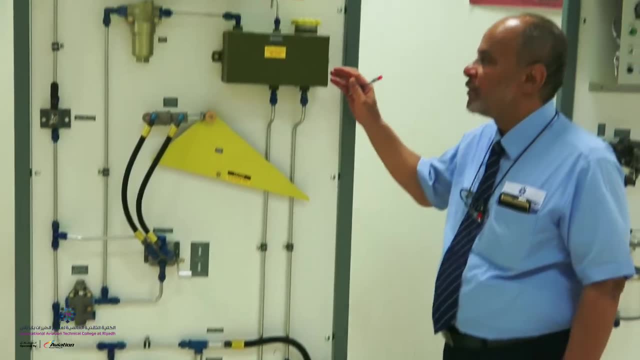 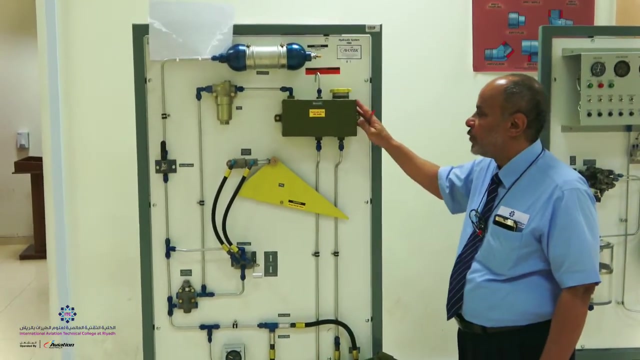 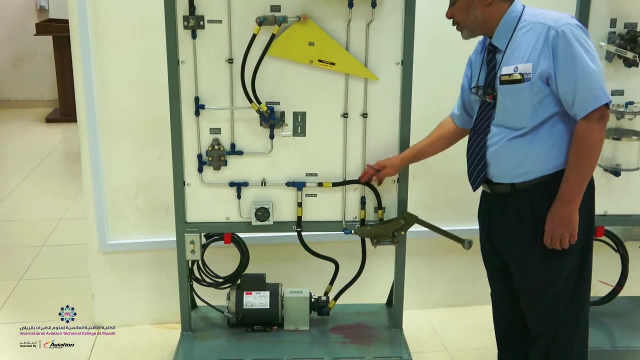 And we have a unit here known as accumulator, as an emergency backup Hydraulic system. It's composed of four main parts. Number one is known as the suction feed. It is where the fluid is being sucked to the pump via the lines and the hoses. 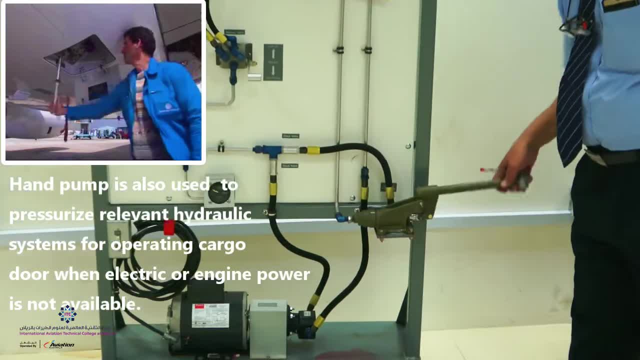 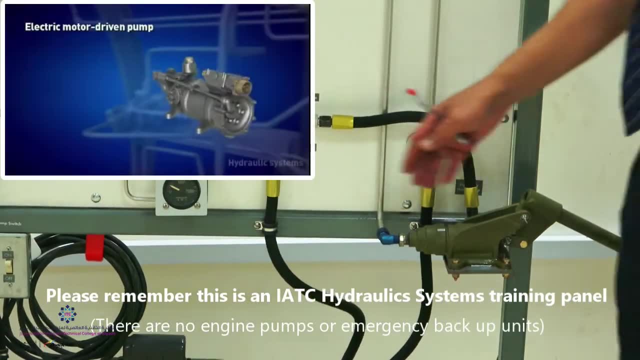 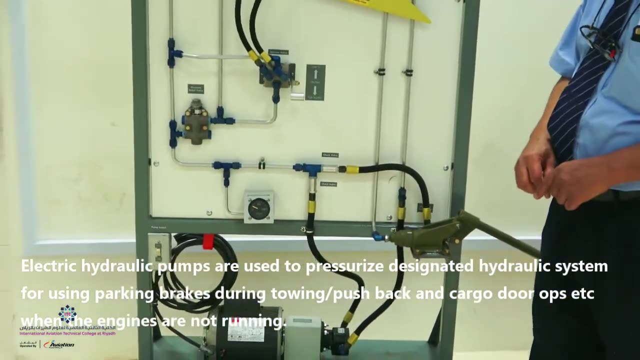 Pumps here are shown: the manual pump. It is used for maintenance purposes usually, And also we have an electric pump shown here. And also we have an electric pump shown here Which will pressurize the system. And also there is a third pump known as EDP. 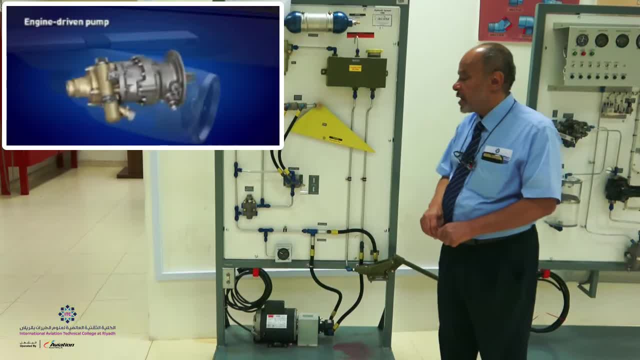 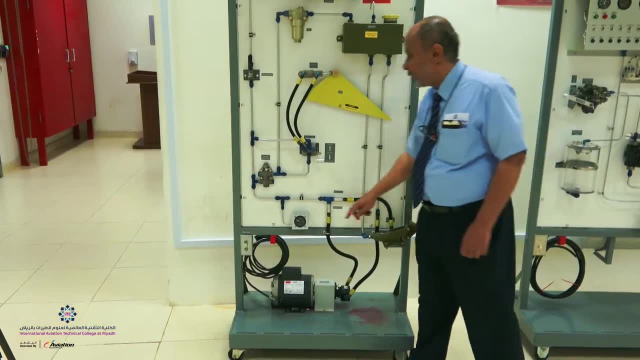 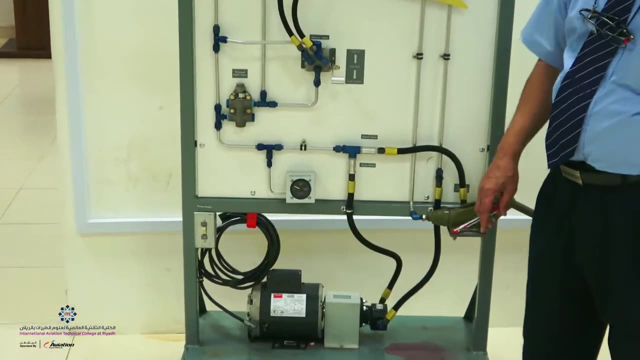 Engine driven pump attached to the gear box of the engine, Any or either pump. once it is working, it will pressurize the system. And that takes us to part number two, the pressurized manifold. Pressurized manifold will carry the fluid and the pressure.